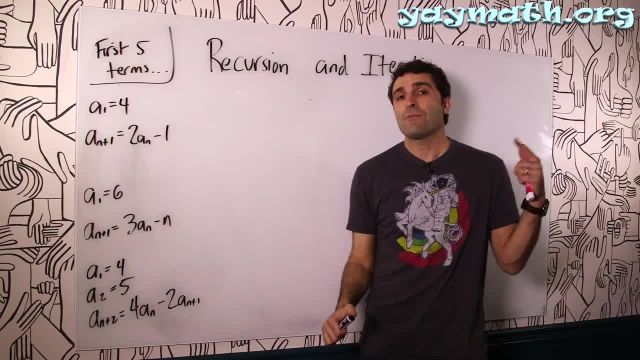 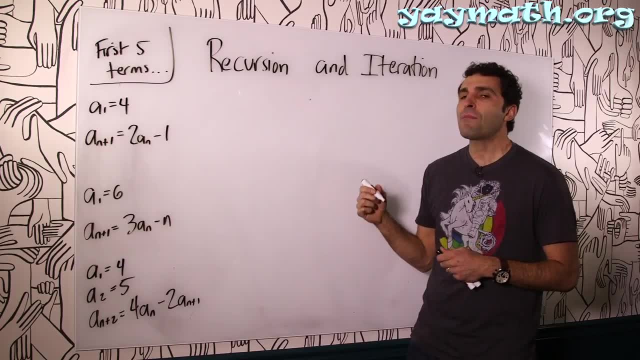 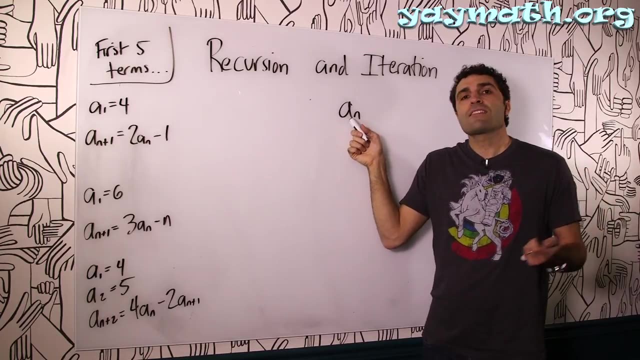 so bad and basically see it the way the authors of the book see it. That would be my primary goal today. all right, And I hope I meet that goal. I hope I accomplish that on your behalf. Let's talk about AN. okay, This is a sequence called A. okay. You can think of like A1, A2, A3, da-da-da-da-da. 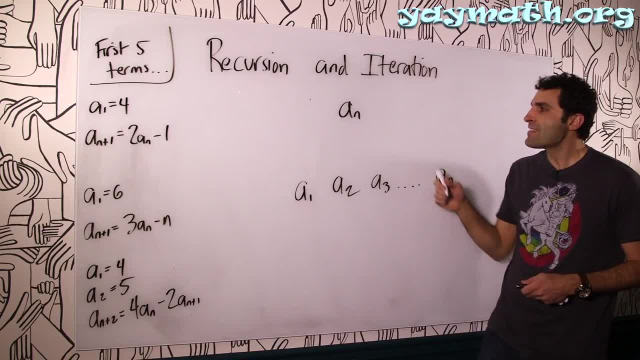 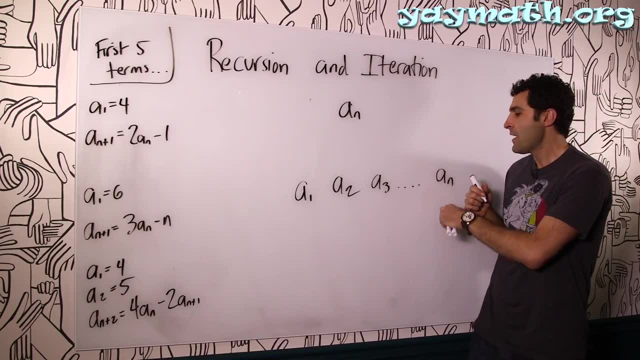 AN. okay, So AN is some sort of term, right, A term that you want to speak about. If it's A3, you're talking about the third term. If it's A4, you're talking about the fourth term. If it's AN. 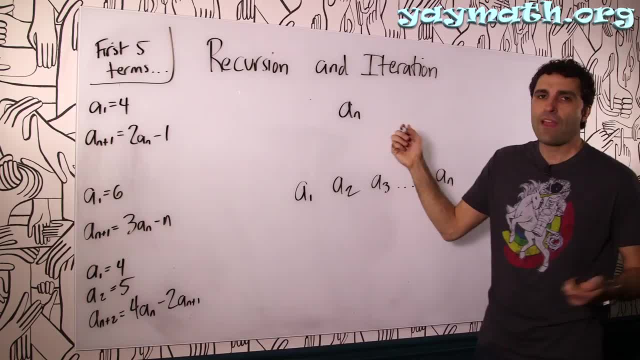 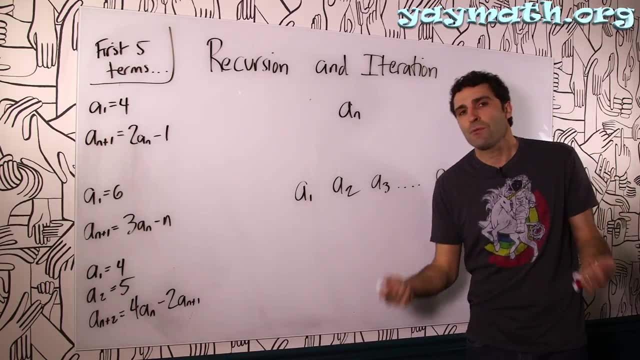 you're talking about the nth term. all right, We can call that. perhaps let's call that the current term, if that makes sense to you, The term that we're talking about. If I said A3,, A3 would be the current term. If I said AN, AN's the current term, Let's put it down: current term. 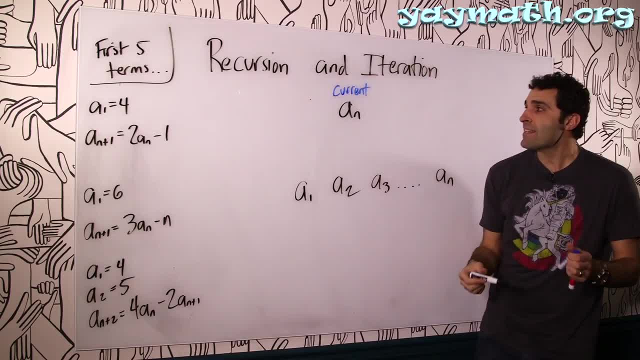 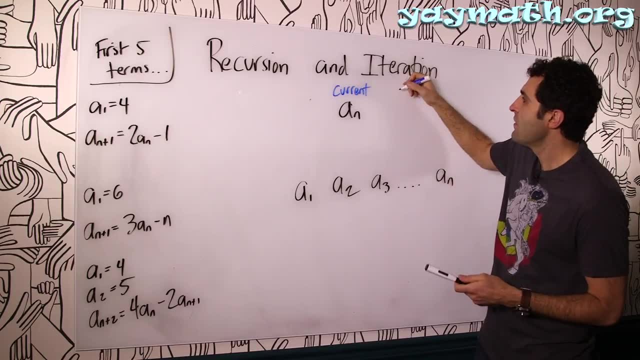 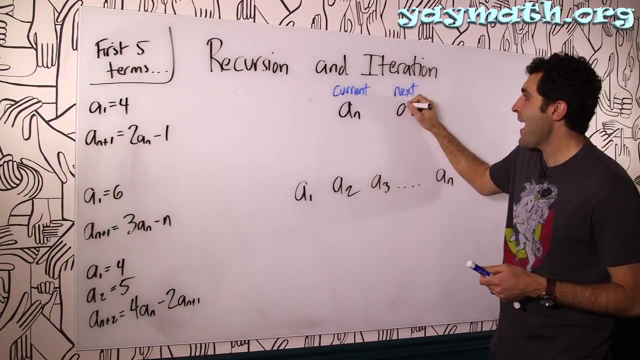 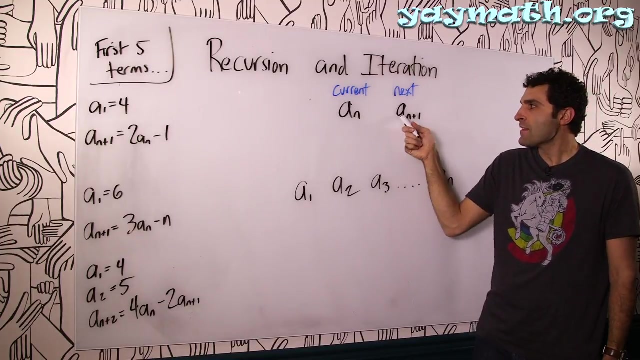 all right. So then it would make sense that the next term- let's put that in blue, save the big reveal- the next term, okay, would be one ahead of this. thus, that is AN plus one. Does that make sense? So it's like, whatever this is, if this was A5, this would be A5 plus one. 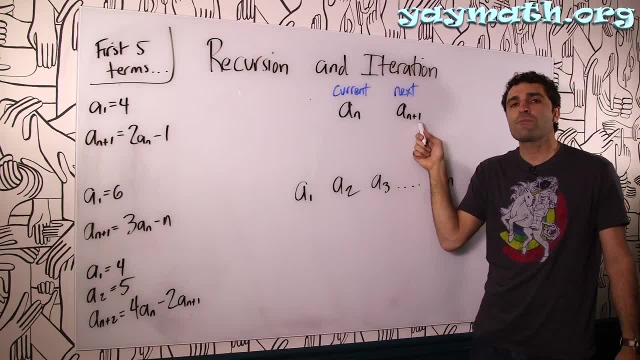 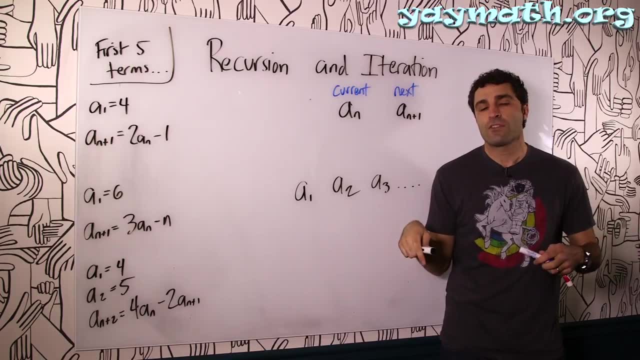 that's A6.. So A5 is the current term. The next term would be A6, which is AN plus one. So from now on, when you see AN, you could think of the current term, whatever term we're on, And if you. 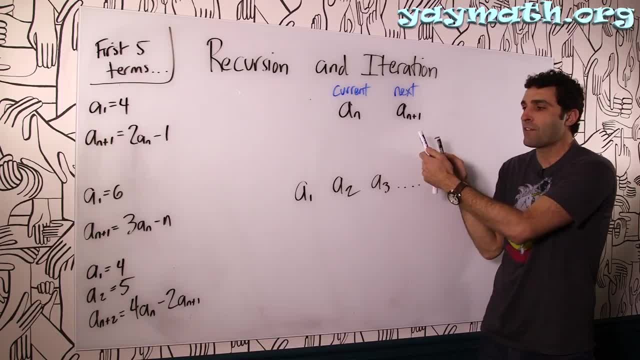 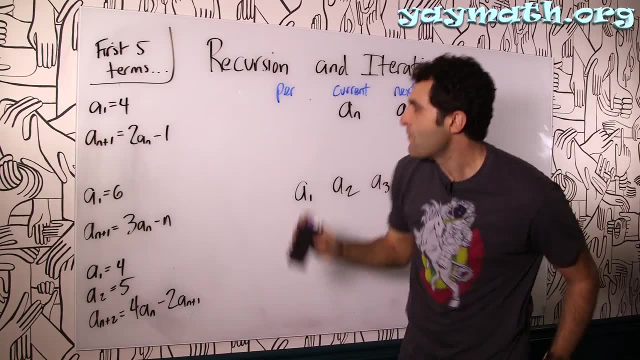 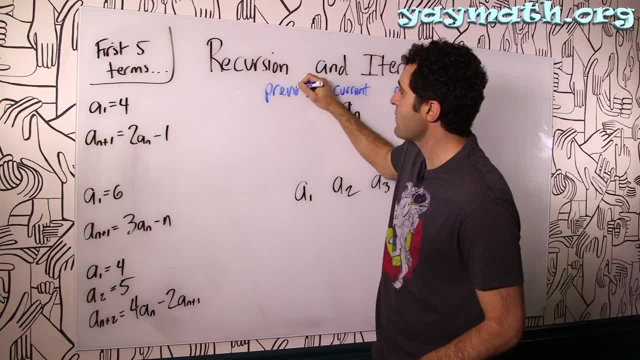 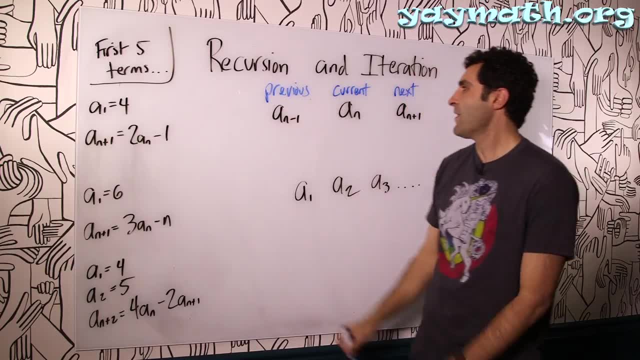 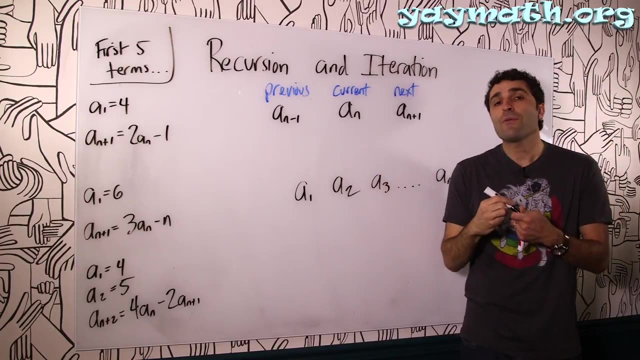 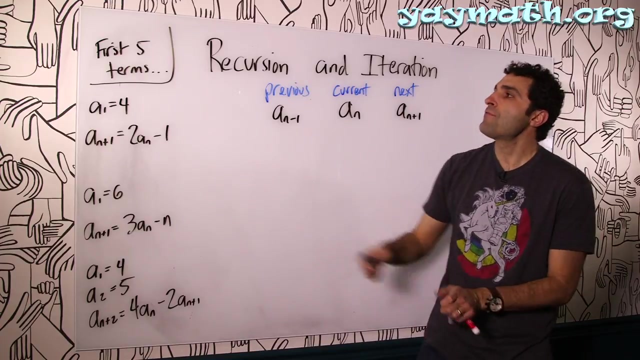 impervious to this confusion. Previous, Say it. There you go. Okay, Current term is AN. Next term, previous term: okay, So now we know the notation. I'm going to leave that up here for a little while. Let's see if we can do the first five terms of this particular sequence. Let's frame the 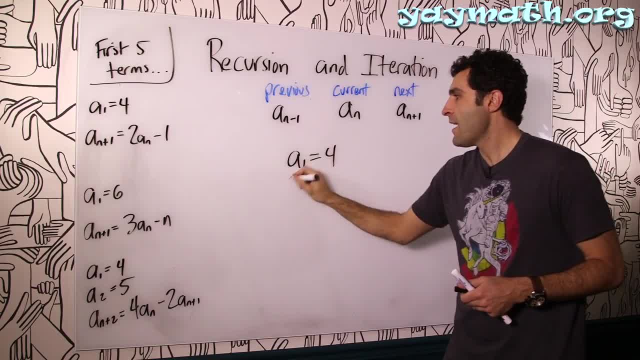 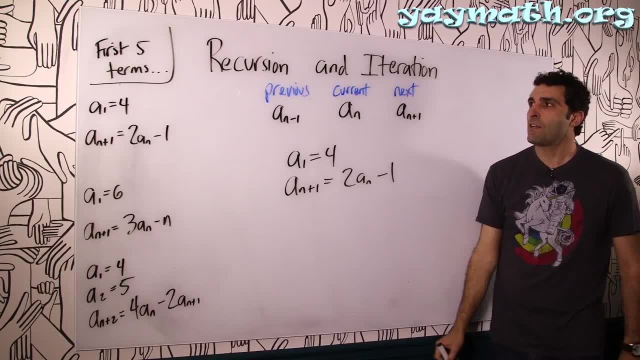 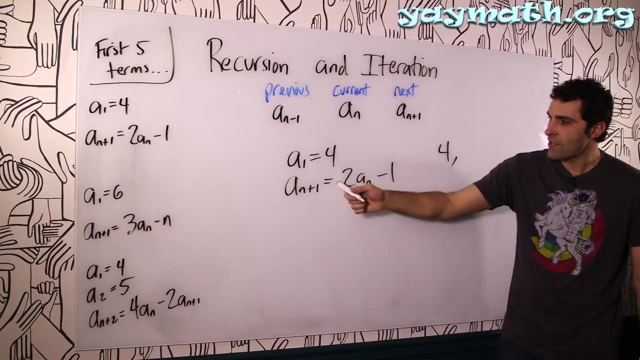 sequence Center A1 is four AN plus one equals 2AN minus one, And we want the first five terms of this sequence Granted. this term is already given to us, So put a four here, four comma. Now look, Look. 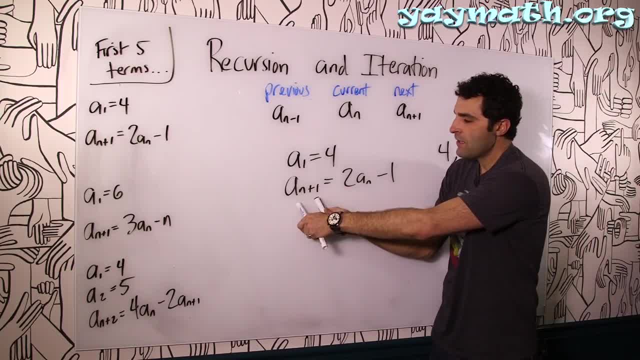 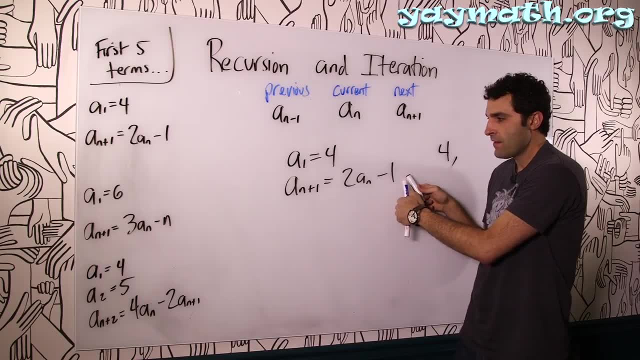 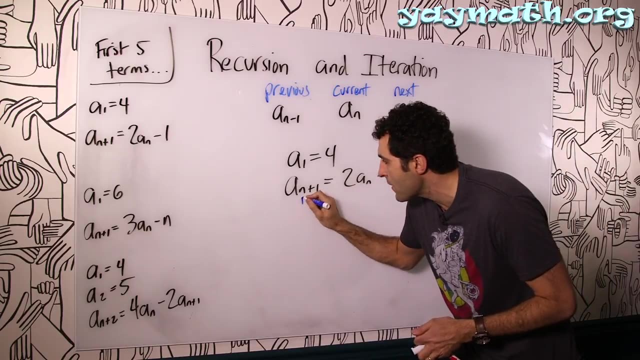 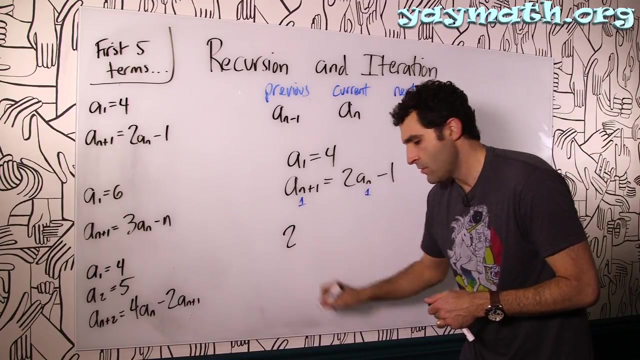 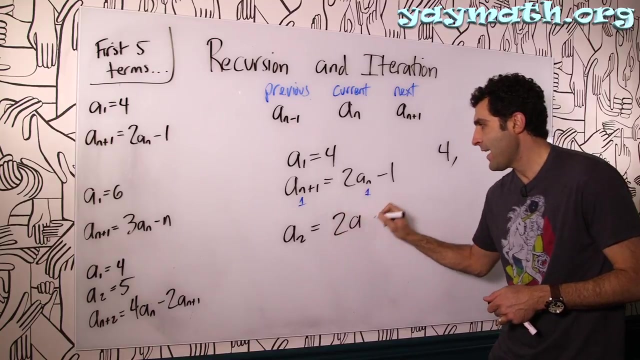 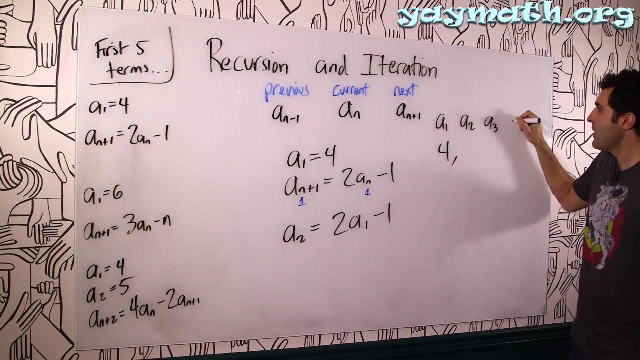 closely. The next term is two times the current term, whatever you're on, minus one. So if you want it to be specific, what if we put a four here? What if we said N was one in this case? If N was one, one would go here, and one would go here, And that would mean A2.. Oops, A2 equals two times A1 minus one. Awesome, This is A1. This is A2.. A3. A4. A5. Right. 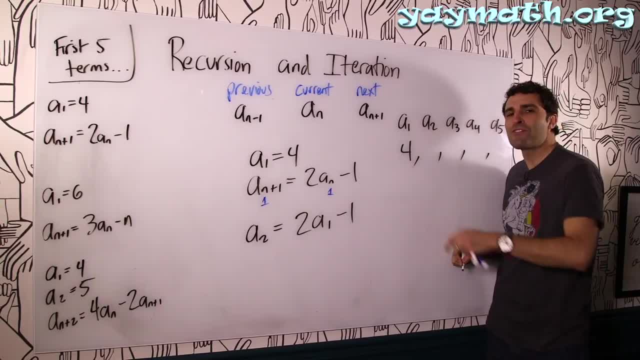 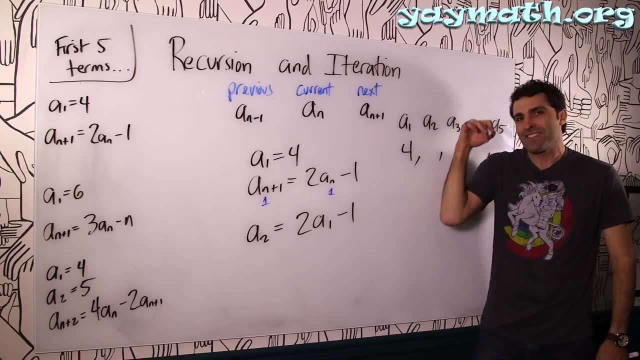 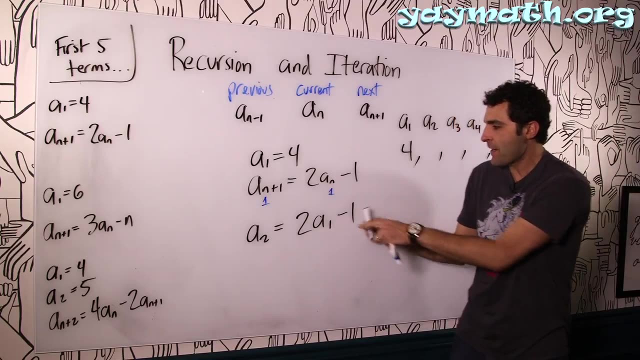 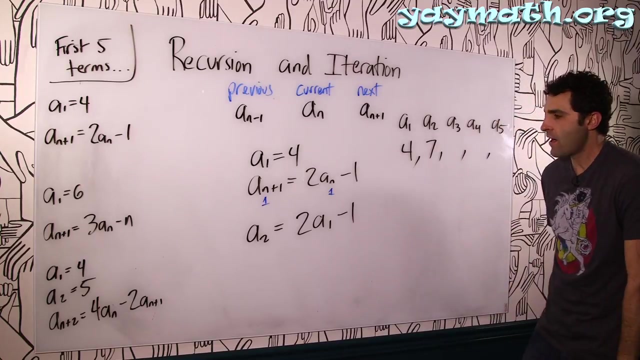 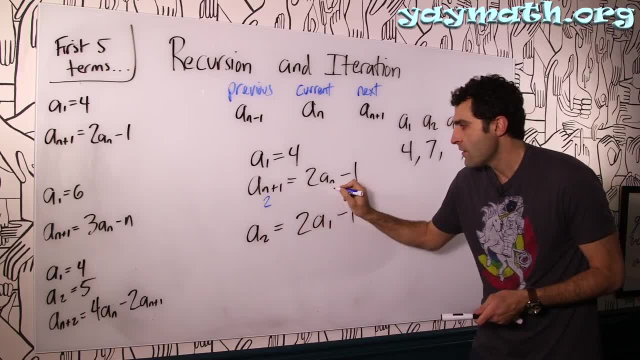 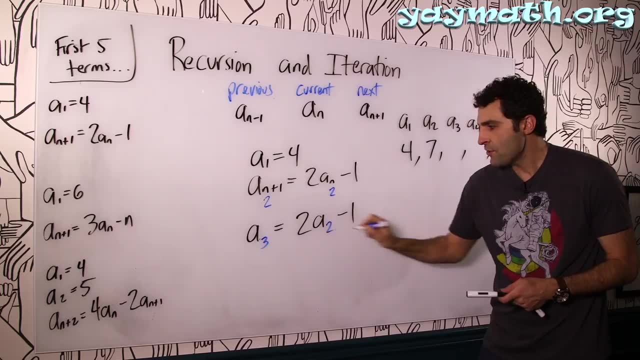 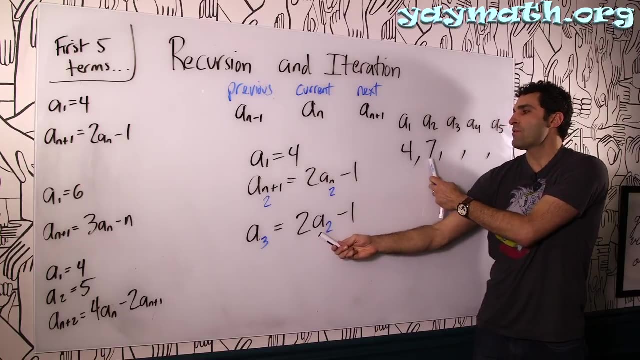 Okay, Okay, Two and two here. So that would mean a two plus one, that's A3.. Two times A2 minus one, Let's find out. Cool A3 is here. Two times A2, which is two times seven, is fourteen. 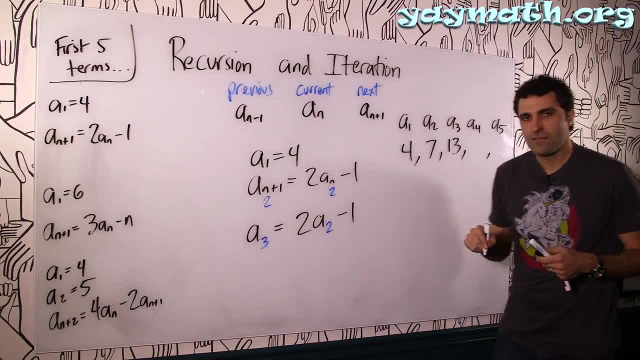 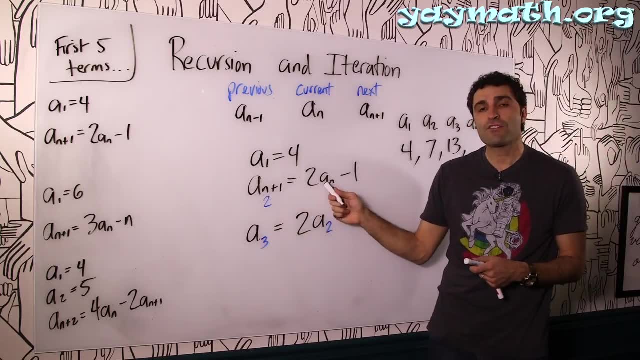 Minus one. Thirteen Jaffeel. did you get the feel for this? So, basically, all it is is: The next term equals two times whatever term you're on, minus one. Let's do it. The next term is two times whatever term I'm on. 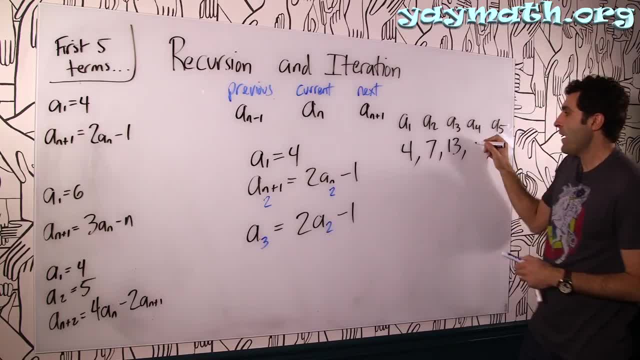 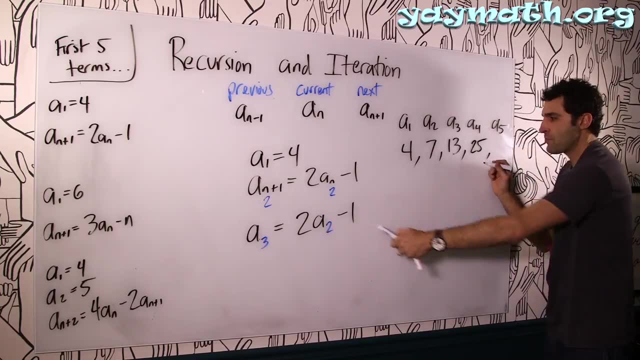 two times this: 26, minus one, 25.. The next term is two times whatever term I'm on: two times 25, which is 50, minus one, 49.. That's all. it is okay. That's all it is. 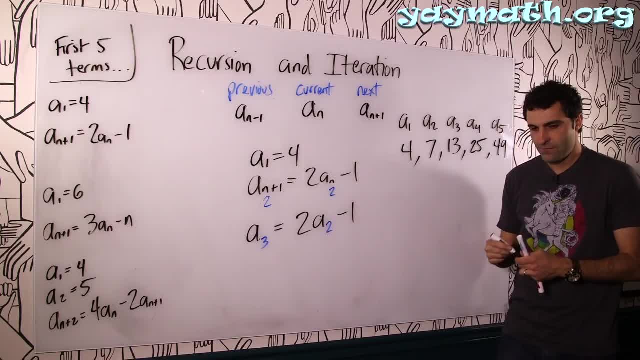 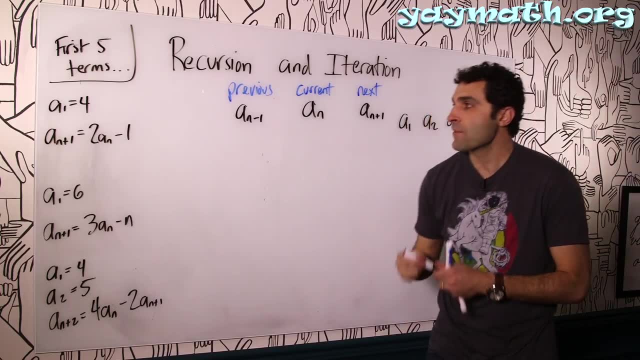 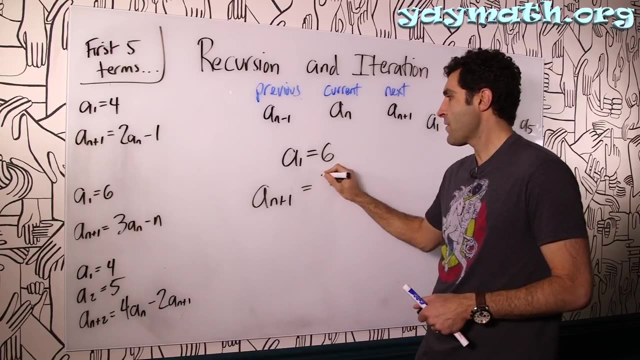 Next term two times current, one minus one. You'll see it's the same over and over. All right, we'll take this off. We want the first five terms again. I'm bringing that over. A1 equals six AN plus one equals three AN minus N. 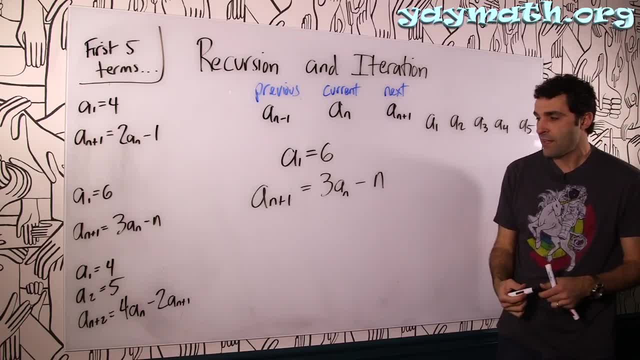 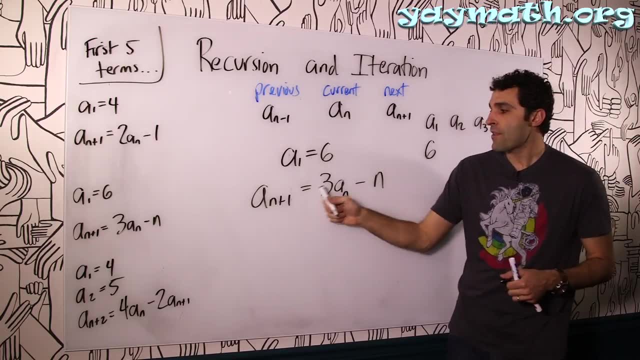 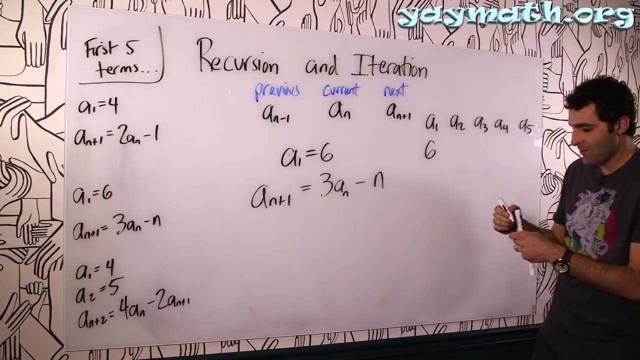 Okay, I'm gonna take a risk, I'm gonna jump straight into the process. okay, A1 is six six. Now the next term equals three times the current term minus what N is at the time, Which is kind of weird, right. 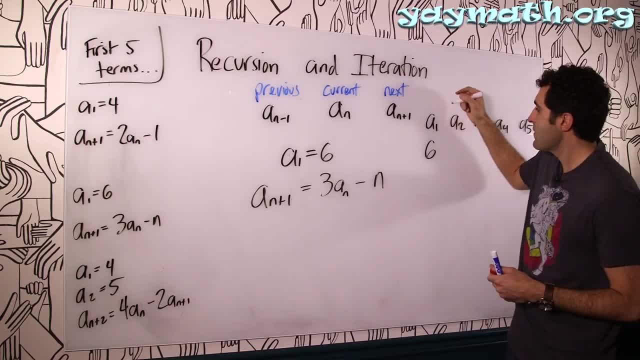 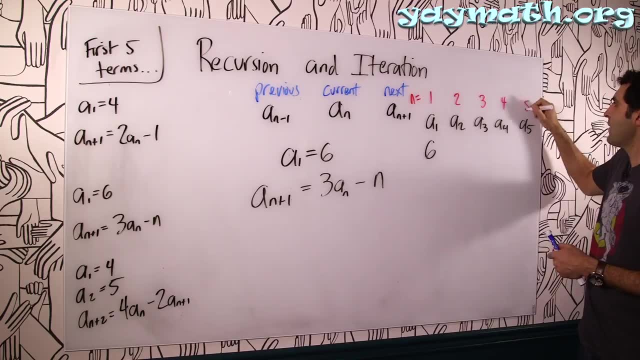 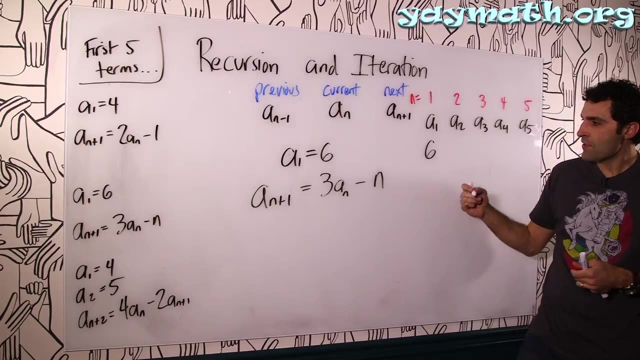 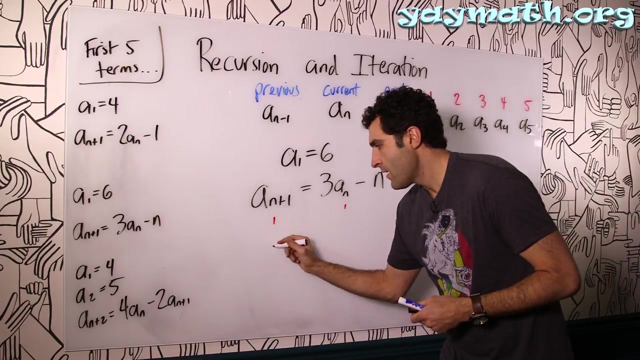 Let's put down N here. So in this case let's go. N equals one, two, three, four, five. look at that, All right, many layers. So let's say: if N was one, okay, That would lead us to A2 equals three times N. 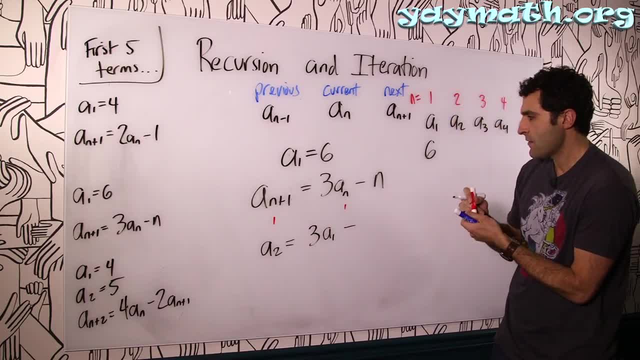 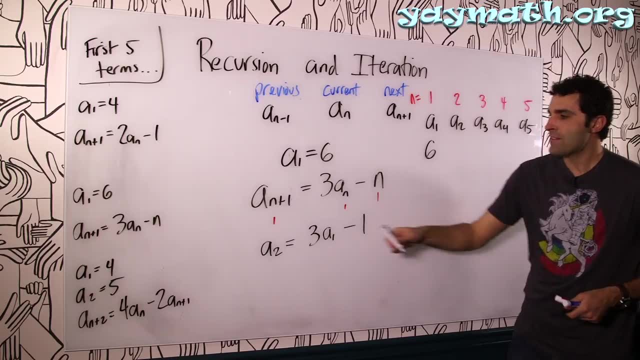 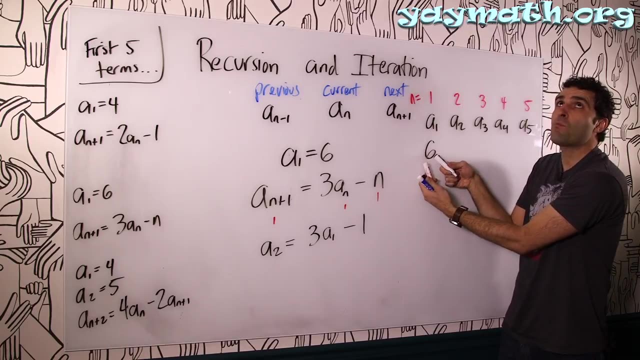 Three times A1 minus- oh, I forgot to put one there- one Minus one. Here we go. A2, this guy is three times this guy: 18, minus one, 17.. Okay, here we go again. 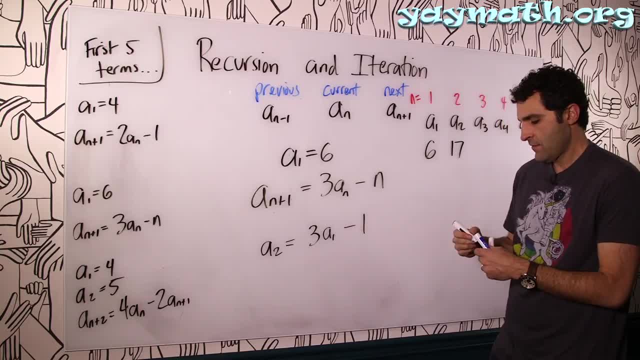 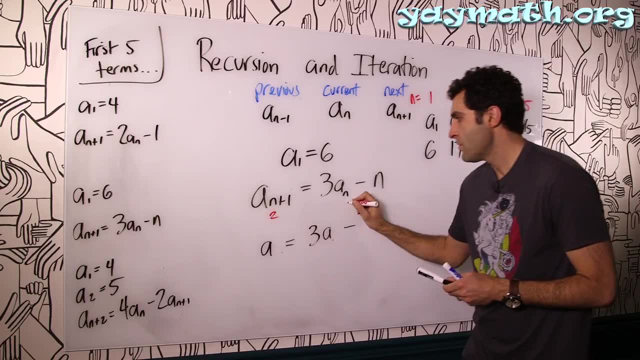 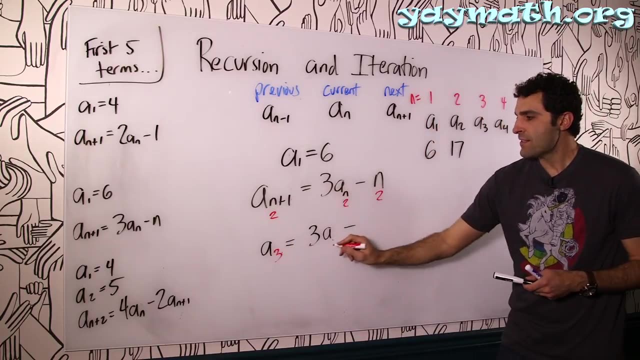 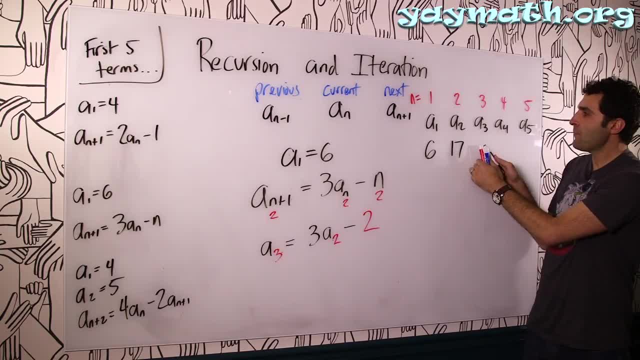 Isn't that crazy. All right, let's do it. A3, this one is three times this. Three times 17 is 51.. Minus two is 49.. All right, Ready to do it? I bet you could jump in with me. 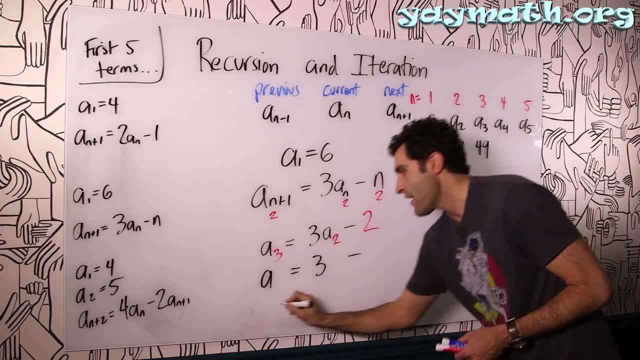 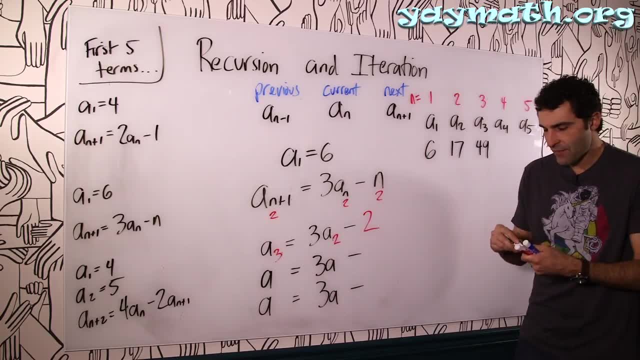 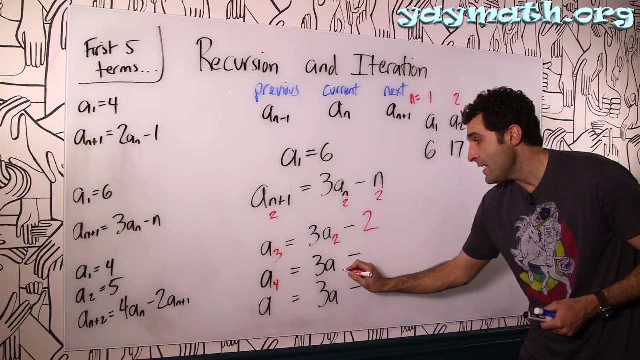 Let's try this: A equals three minus. A equals three A A minus. Okay, let's have a little fun with the pattern. This would be a four. This would be a three. This would be a three. See it. 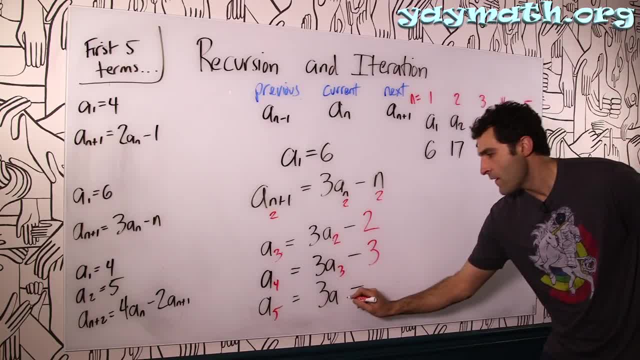 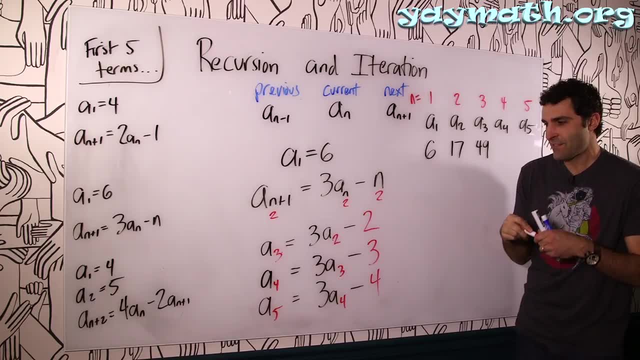 Two, two. This would be a five. This would be a four, Four. This would be a four, Four, Four. Got to go a higher octave because it's the last one And then Okay, so let's try it. 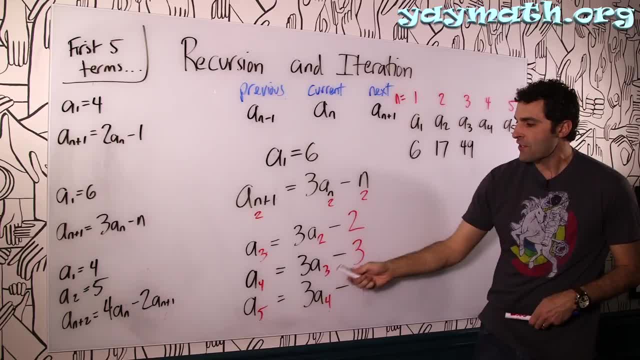 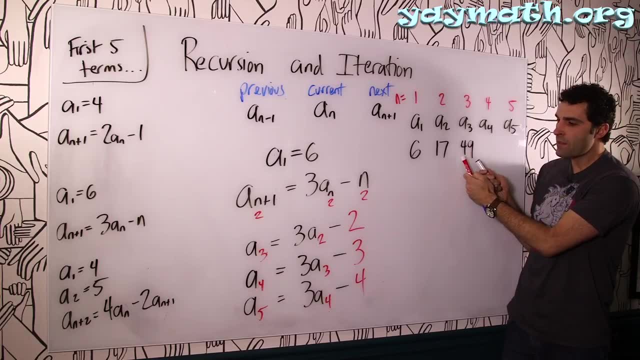 A4, the next term equals three times the current term, minus the number N that you're on. It's kind of cool. All right, let's see if we can bang this out. Three times 49 is 147.. Minus three is 144.. 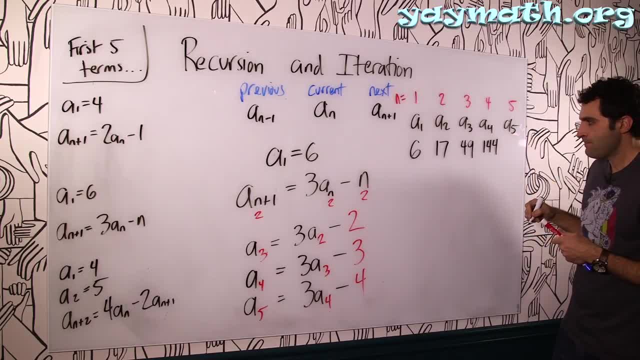 Pop it in: Good Yeah, three times 49.. It's like three times 50 minus 111.. That's 147 minus three. All right, here we go. The fifth term is three times the fourth term, Three times this is. 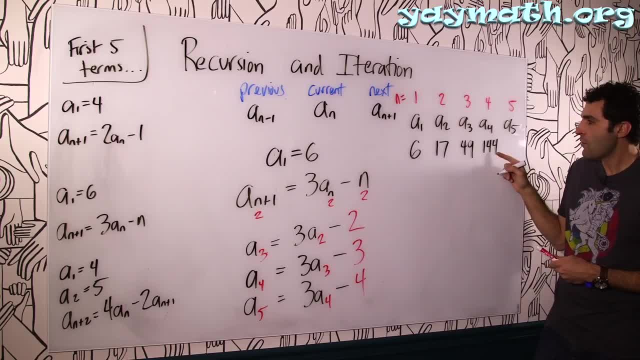 Oh, here we go: 300 plus three times 44.. 44 is 88. And then another 44 is Ah, bailing out, Bailing out. Got to rely on tech sometimes. Okay, let's see, Let's see. 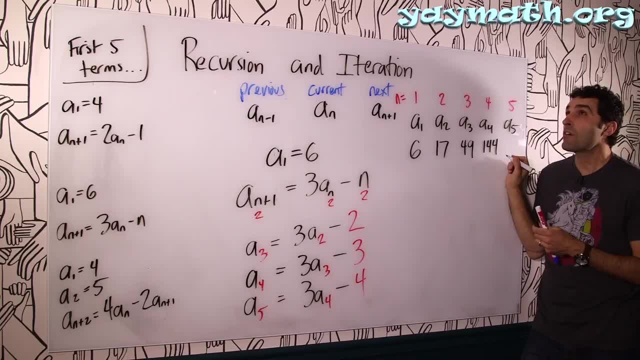 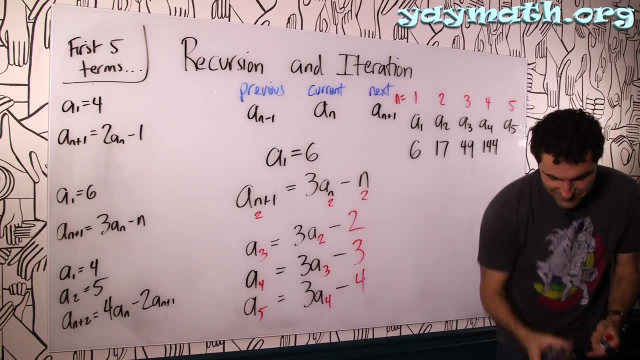 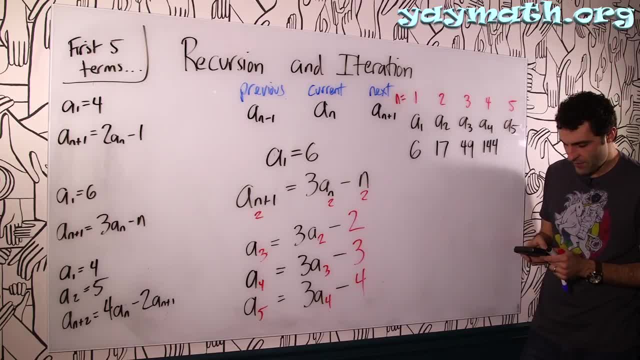 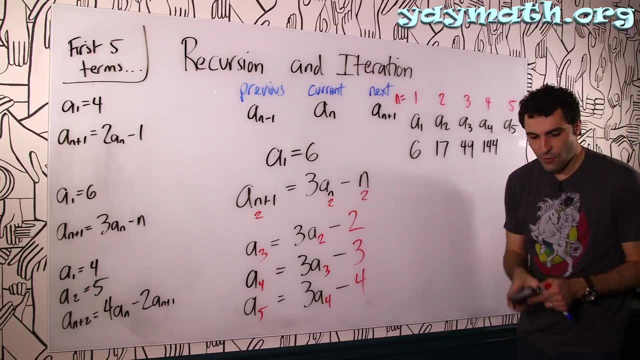 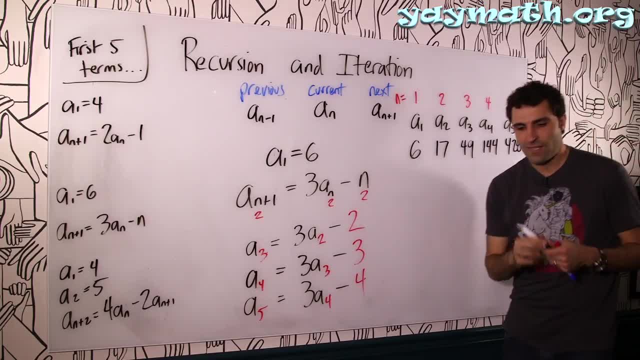 Let's see, Come on, We have come so far. We have come so far. We're going to have to rely on tech. sometimes 144 times three, 432 minus four, Four, twenty-eighths. Okay, There you go. 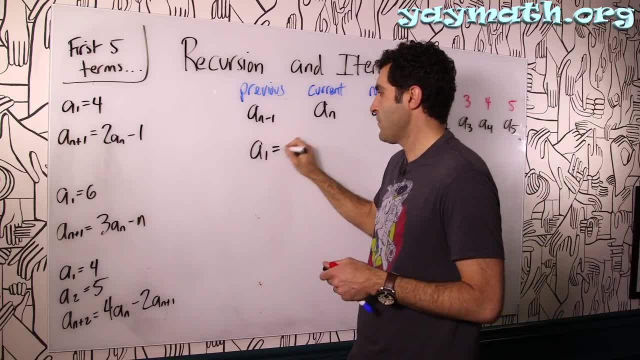 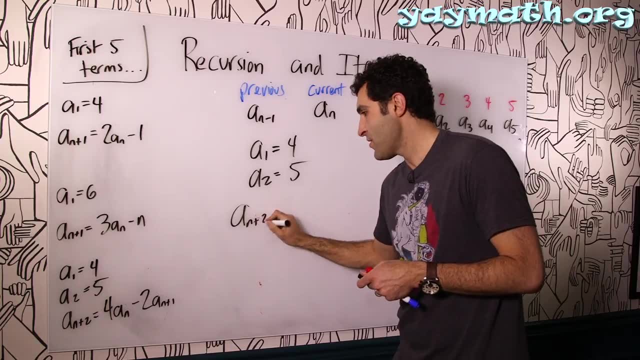 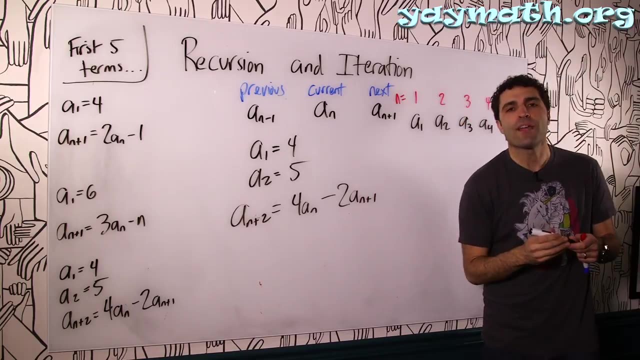 That one's done, Let's do the first five terms of the next guy. Let's see if we can get the language even more. A1 equals 4.. A2 equals 7.. That's right, That's right. 5 a n plus 2 equals 4 a n minus 2 a n plus 1.. Back to the original point. The original point is: 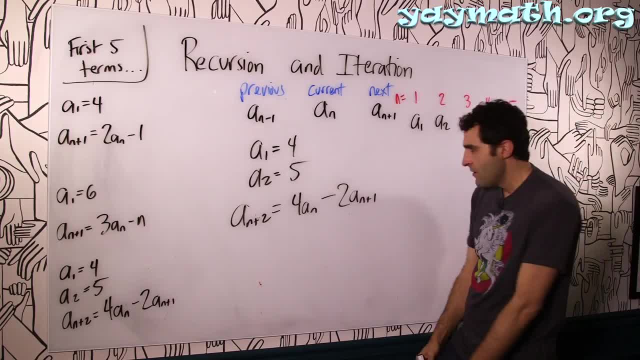 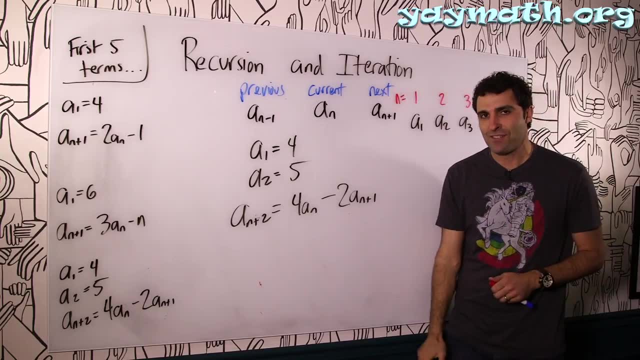 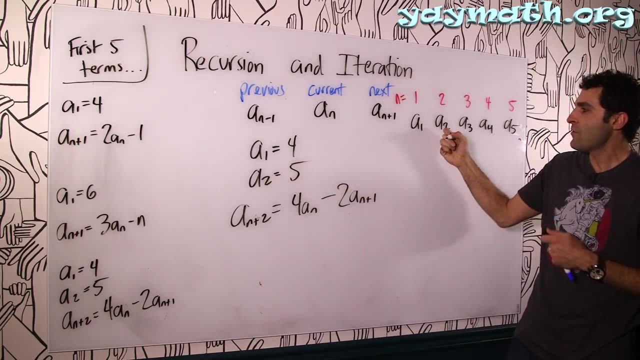 when you look at this all together, that's what goes through my mind, That's how I feel, looking at this as if I'm seeing it for the first time. okay, But we don't have to be bound by that anymore. This means first term. This means second term. We're already two-thirds of the way there. 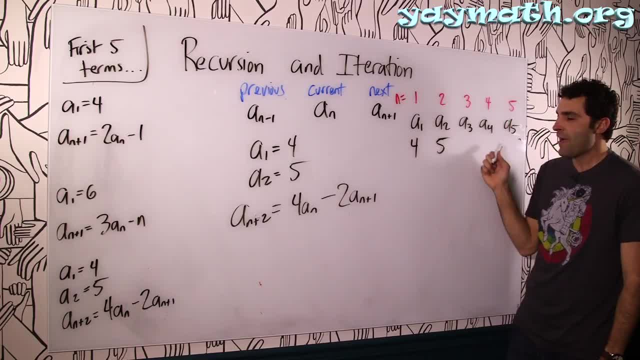 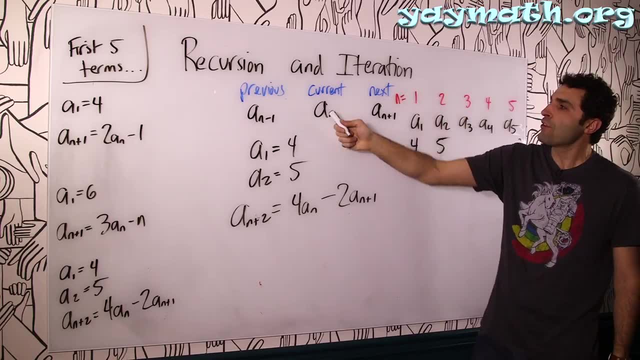 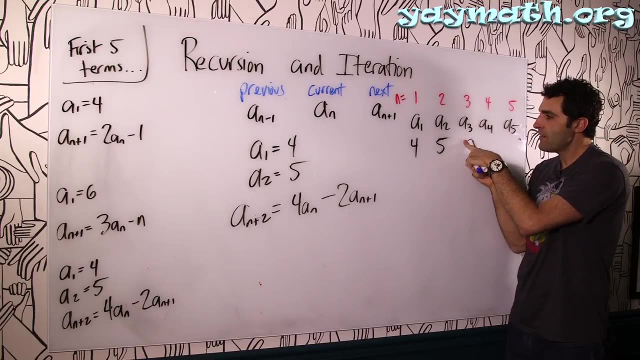 Four, five or two-fifths of the way there. Four and five Next. this is the term next after the current. So two ahead, Not one ahead, but two ahead. So let's have some fun with it. Two ahead equals four times whatever. the current term is Four times this. 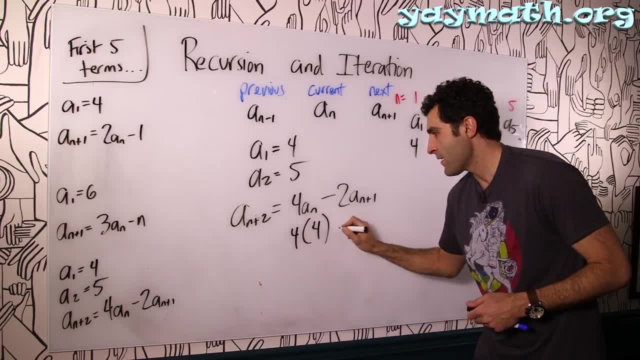 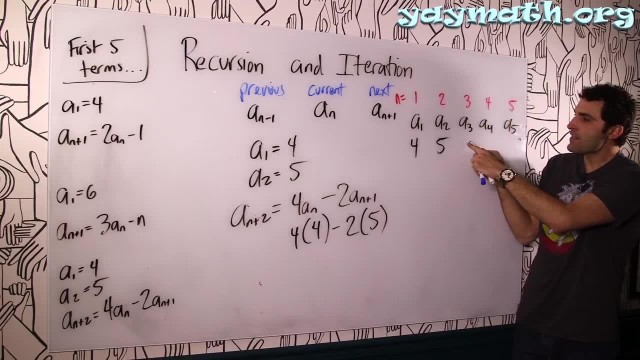 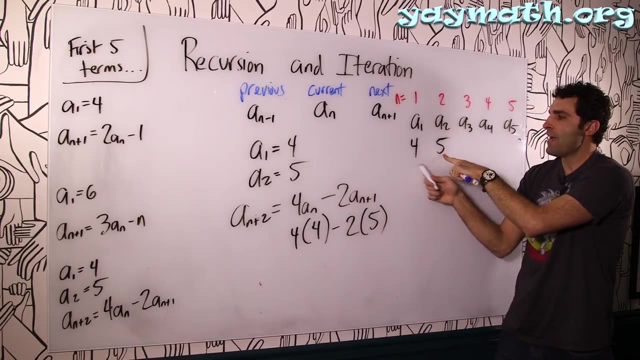 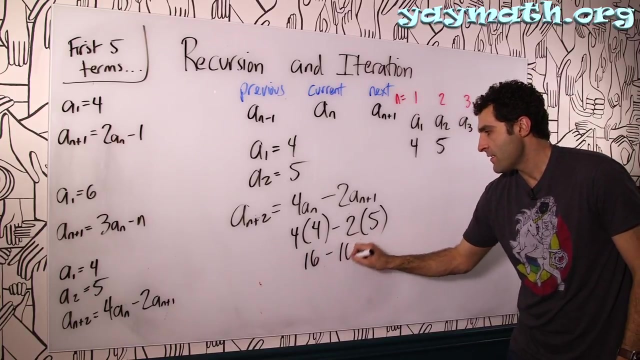 Why not? Let's put it all in black: Minus two times one ahead. See that This one, when you're two ahead, is the same as four times the original, one minus two times the one ahead of original. the next term, This is 16 minus 10.. That's six. Whoa interesting. Will that happen again? We'll. 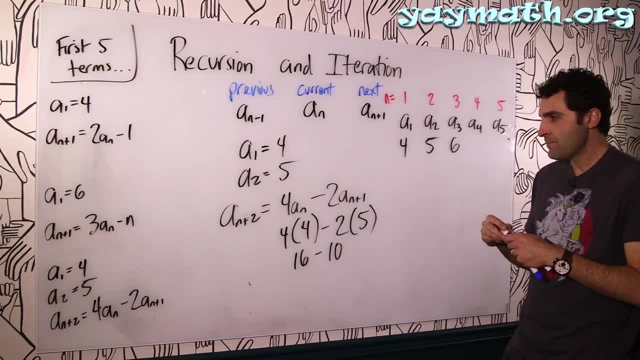 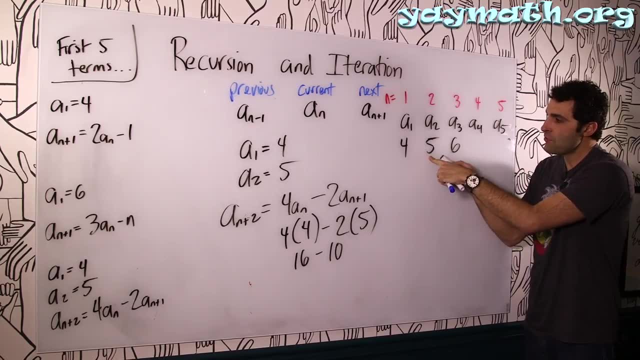 find out. So let's try the next one. The one over here would be four times the original one. we're starting with right, So we're like two ahead of this, all right. I want you to think in those terms. now, Here we are, two ahead of original, okay, Which is what we want. So we have four. 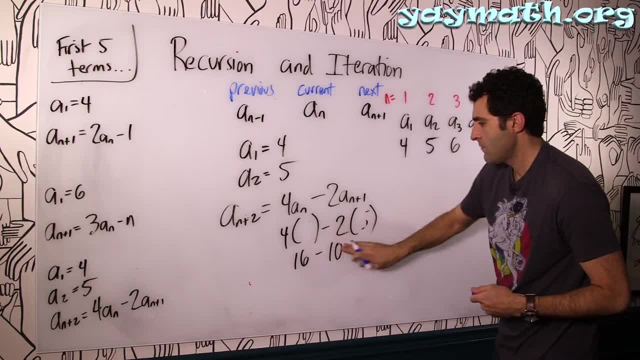 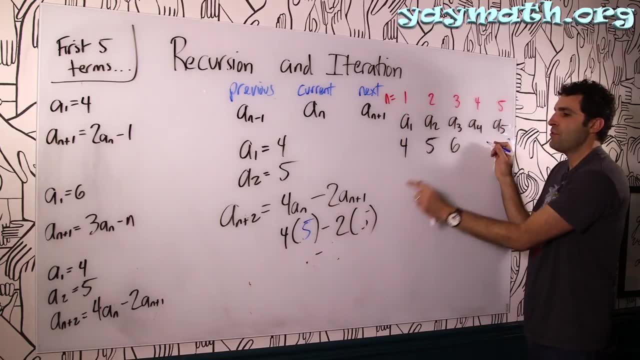 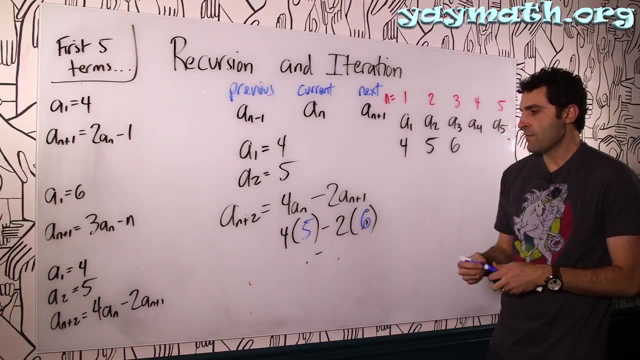 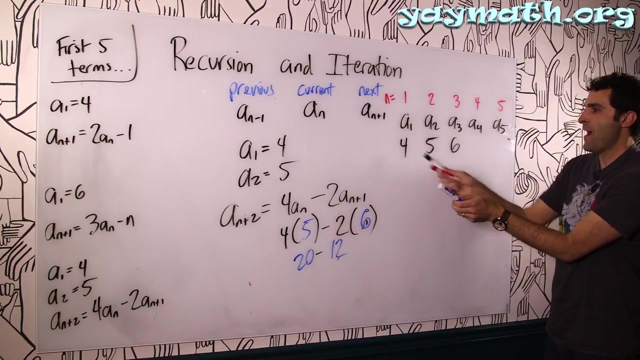 times. Now we can put a little color in. Okay, Four times original, that's four times five Minus two times one. ahead of original is two times six. Let's see if it happens, This becomes 20 minus 12.. Oh, couldn't keep it up. Eight, I was looking for that pattern. There's eight. 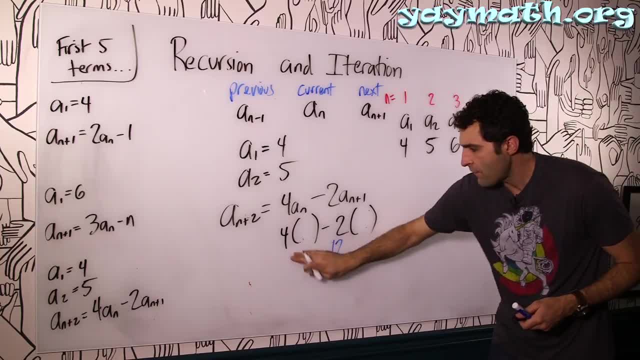 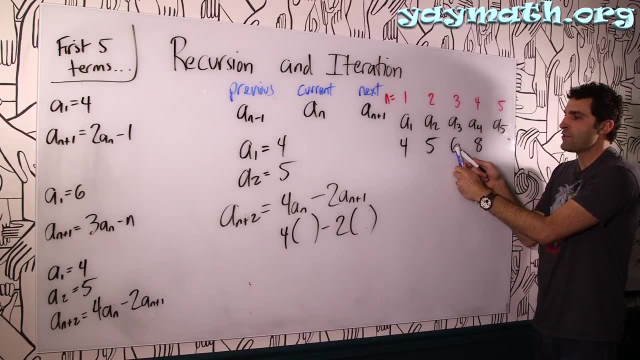 And finally, off, off, off, off, off, And we'll get them in. All right, This one is two times the original plus, Oh, four times that. one Excuse me, Four times that and two times that. Let's put it in Four. 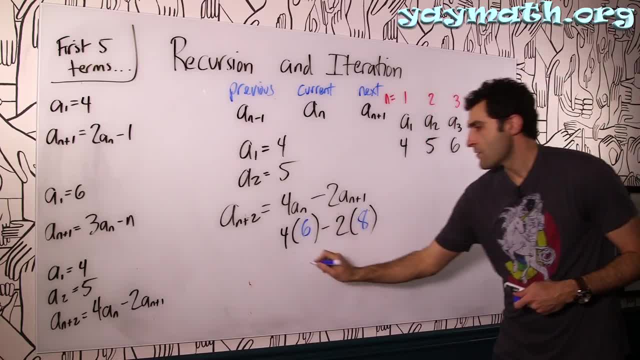 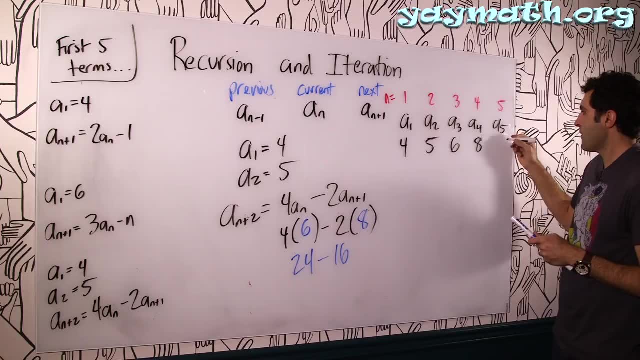 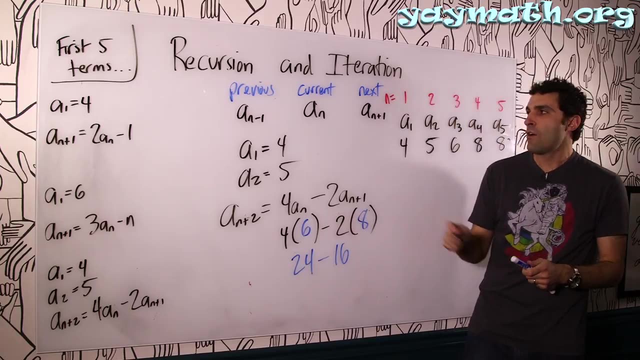 times six, two times eight, 24 minus 16.. How about that? Another eight, Another eight. Okay, I hope that makes sense right? Think in terms of current and next and previous. One ahead, two ahead. Therefore, this would be two back. 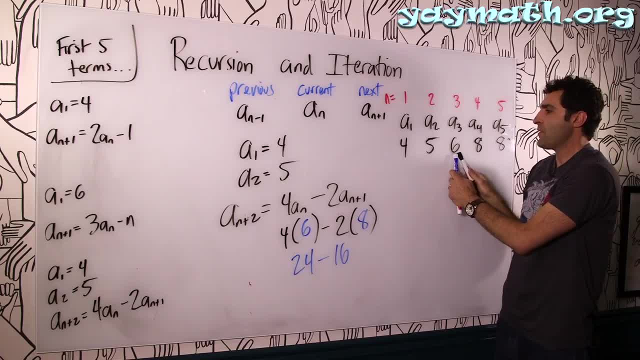 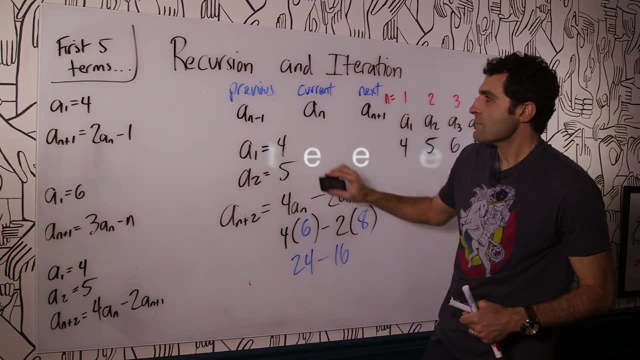 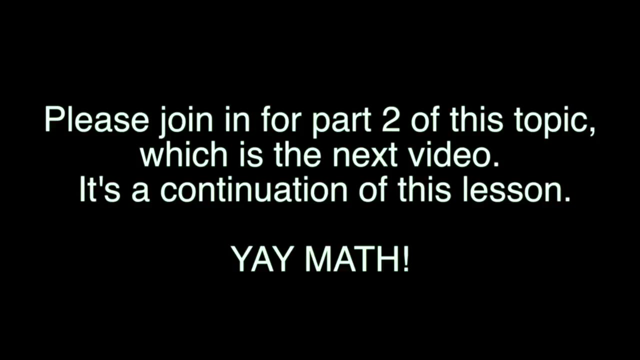 AN plus two over here. That's two back. This is AN plus two. This would be AN. This would be AN plus one. All right, Good job, Let's go. Okay, I'm going to take all these off now. Part two will be. 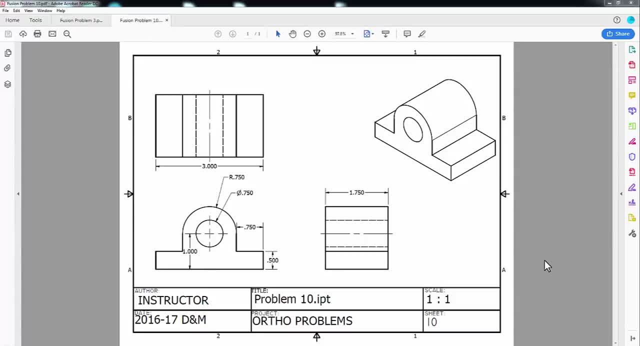 In this video we're going to talk about how to read an orthographic projection, also known as a multi-view drawing, On the screen right now you'll see a basic common orthographic drawing. The definition of an orthographic drawing is projecting multiple views of a three-dimensional object. in 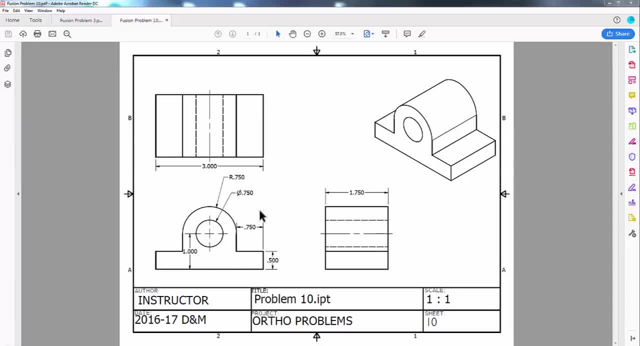 separate two-dimensional drawings. You'll see here in the upper right-hand corner of the sample drawing that you have a three-dimensional view. More specifically, that's known as an isometric three-dimensional drawing. In the other left-hand corner you can see you have multiple two-dimensional 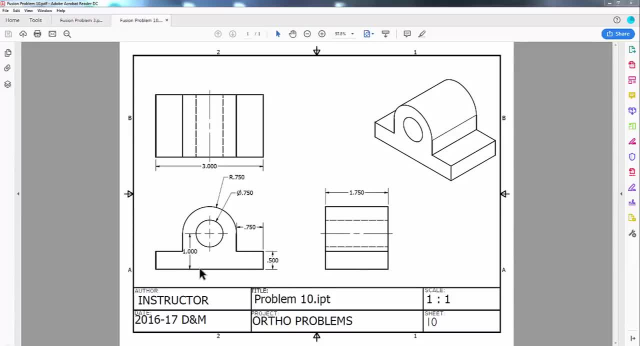 drawings. In each of these drawings, you can only see two dimensions, So in this view, you can only see width- side-to-side- and width. In this view, you can only see width, side-to-side and width. In this view, you can only see width, side-to-side and height. In this view up here, the top view, you can see the width and you can see the depth. We're going to explain how to read these and gather measurements off of them so that you can learn how to use these to make items in 3D modeling.